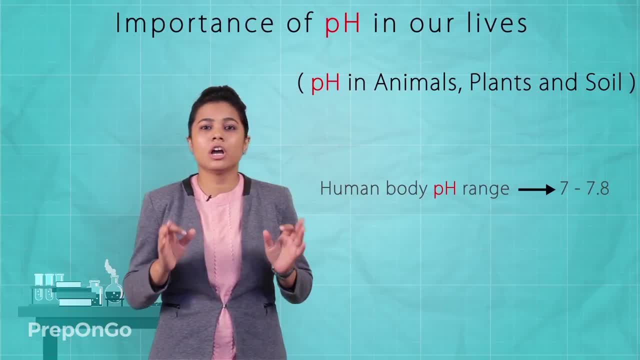 Now this narrow range of pH is essential for the proper living of the bee. 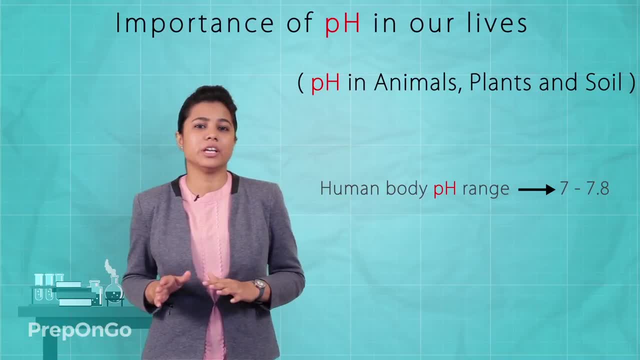 Now if the pH is more acidic or basic, then it can cause a lot of pain, irritation and many abnormal activities in the body. 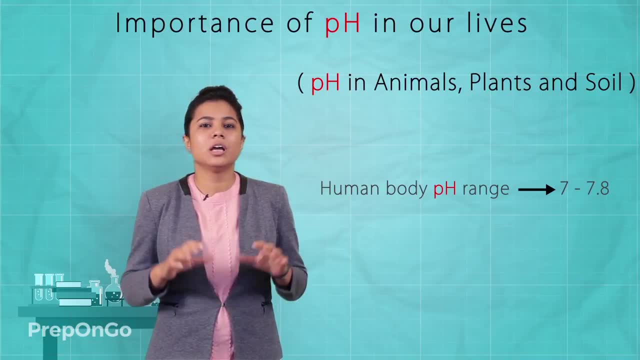 So these pH has to be maintained by eating healthy food. 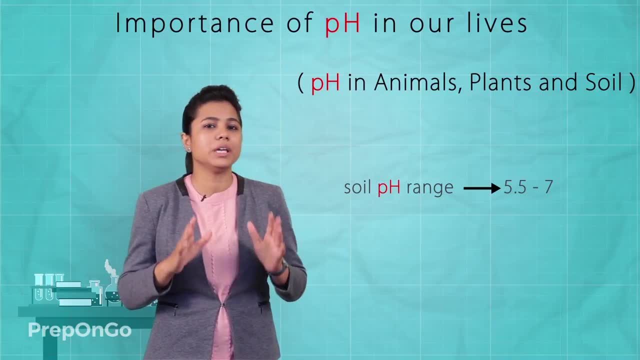 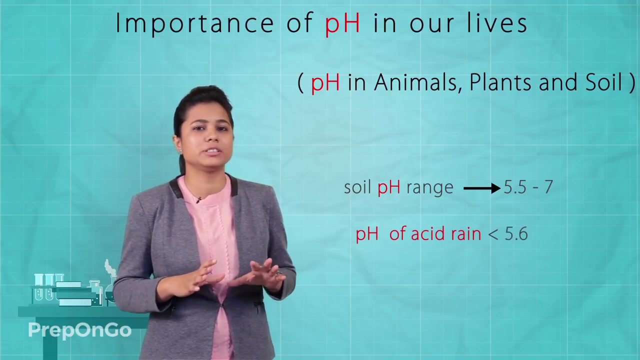 Now soil also requires a minimal pH of 5.5 to 7. This is because it provides a proper growth to the plants. Now sometimes this pH lowers because of the acid rain. Now the acid rain has pH less than 5.6 and that is why it is called as acid rain. 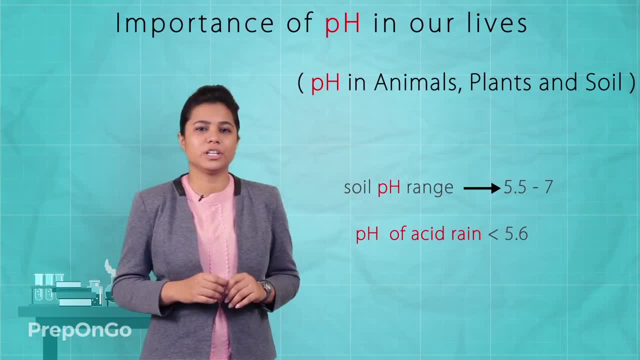 These acidic rains disturbs the pH of the soil. Now when the soil becomes acidic, it can be neutralized with the pulverized limestone. The acid rain also affects the rain river water and makes it difficult for the aquatic life also. 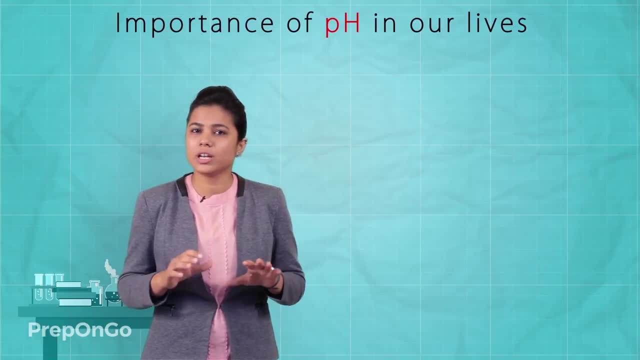 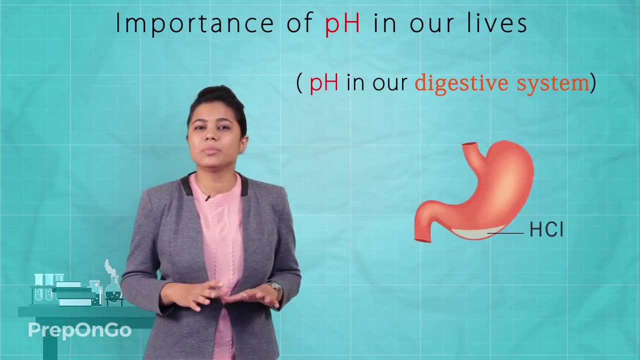 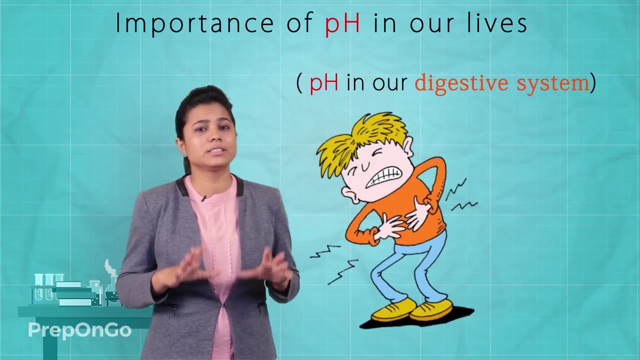 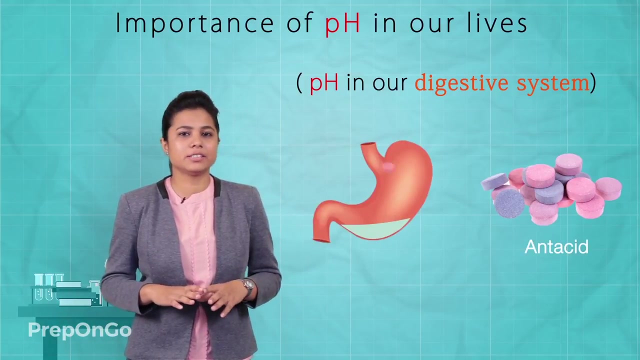 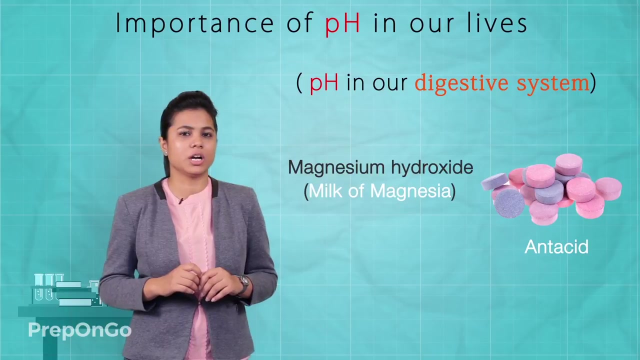 Now let's see what is the role of pH in our digestive system. Now our stomach releases hydrochloric acid for the digestion. Sometimes due to overeating, excess of hydrochloric acid is released in our body. Now this causes pain and irritation. To get rid of this pain, people uses anti acids. Now these anti acids neutralizes the excess of acids. Magnesium hydroxide, generally called as milk of magnesia, are commonly used for the cure of acidity. 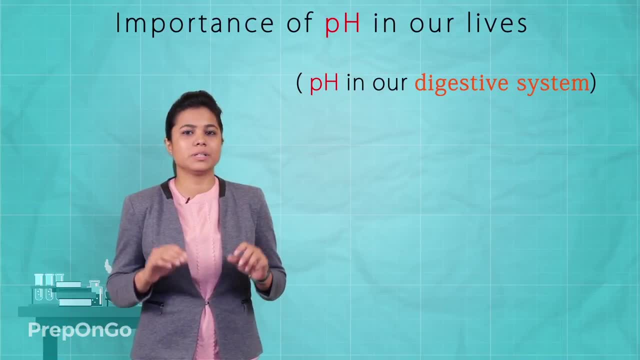 Now the markets are flooded with anti acids but there are also natural remedies such as baking soda or vinegar which are used to cure acidity. 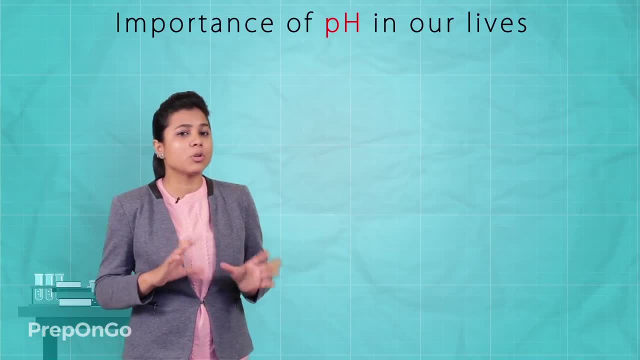 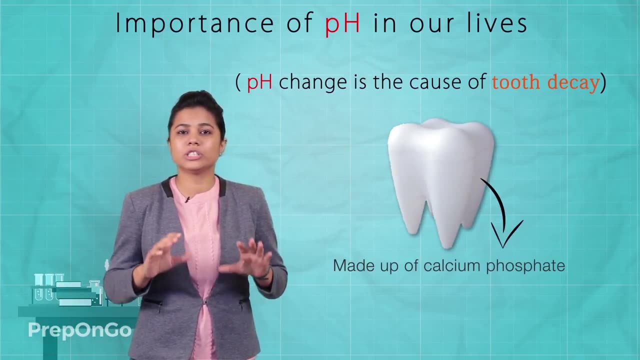 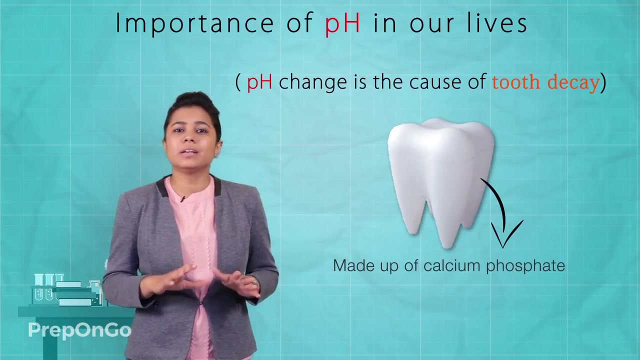 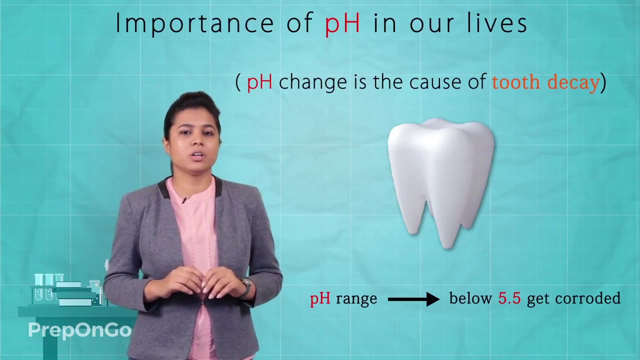 Now the pH also affects or is also involved in the tooth decay. Now we know that the tooth enamel is made up of calcium phosphate which is one of the hardest substance in the human body. Now it does not gets corroded away with water. But it gets corroded when the pH of the mouth is changed. That is up to 5.5. Now this is because the bacteria present in our mouth degrades the sugar and the food particles which are remaining in our mouth.